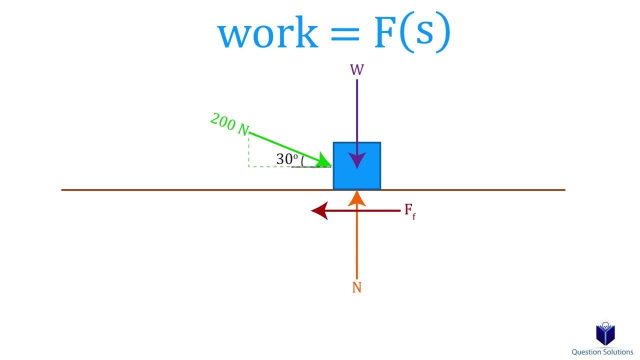 The work done is only done by the x component of this force because, as before, the box does not move up or down. The displacement is in the horizontal direction. so we only look at the horizontal components of forces. So in this example only the 200 cosine, 30 degrees does. 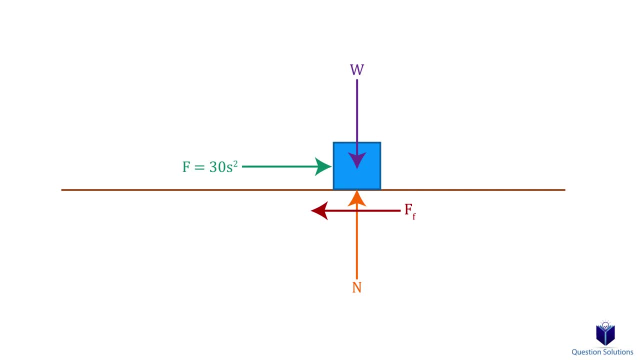 positive work. So the 200 newton force does positive work, while the friction does negative work. Let's now say that the force we apply is not a constant, but rather it's a variable force like this. So this force is dependent on the distance the box travels. Then how do we calculate? 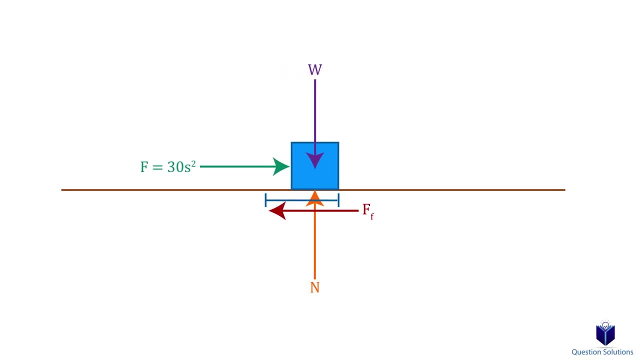 the work. For that we will integrate. Let's say, the box moved 3 meters, So the lower bound starts at 0 meters and the upper bound is 3 meters. We then integrate the force and we can figure out the work that's done. By the way, some books use W to represent work, while I'm 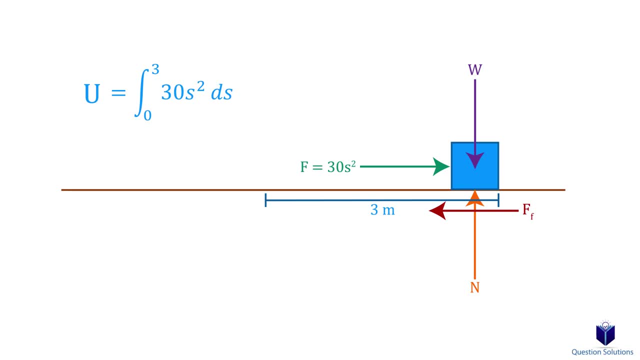 using U to represent work. The unit for work is joules or 1 newton meter. Another thing to consider about work is when it involves springs. Let's continue with our example by adding a spring with a stiffness of 200 newtons per meter. Now let's say our box started like this: 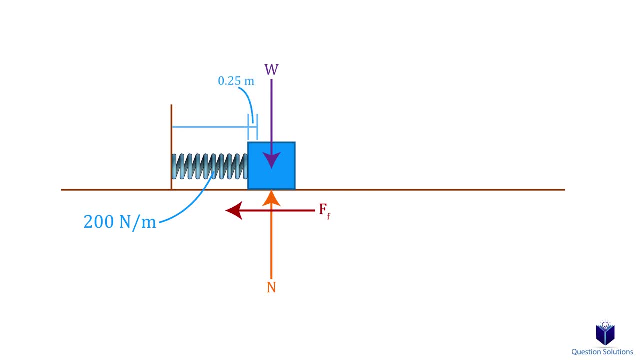 where the spring is compressed: 0.25 meters. Since it's compressed, the spring tries to come back to equilibrium by pushing the box to the right. This does positive work and we see the work done by the is half times the stiffness of the spring times, the displacement of the spring squared. 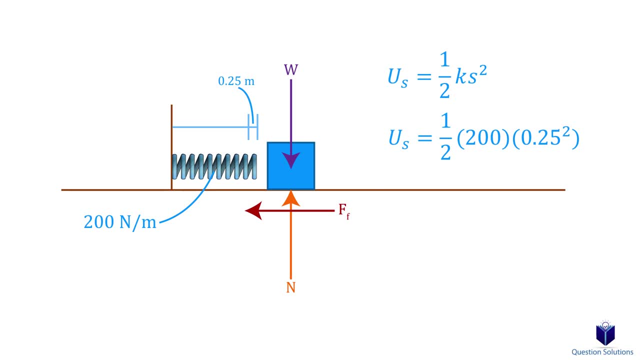 In our case, the work is equal to half times 200 times 0.25 squared. If the stiffness of the spring is not constant, then, as usual, we integrate it from the initial position to the final position. Now, if our box was actually going like this, where it was initially moving to the left, 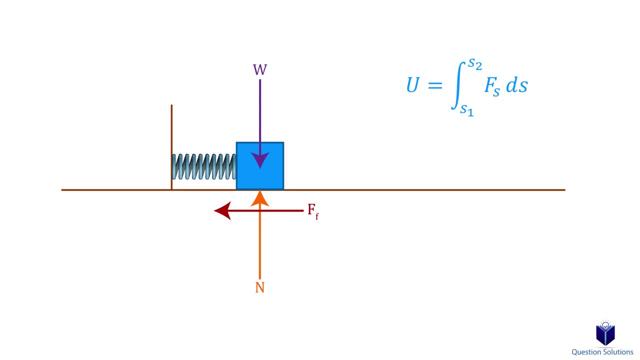 and the spring is now slowing it down, then the work done is negative because it's stopping the block. One last thing to consider about work is with weight. If the particle is moving up or down, then the work done by weight is simply weight multiplied. 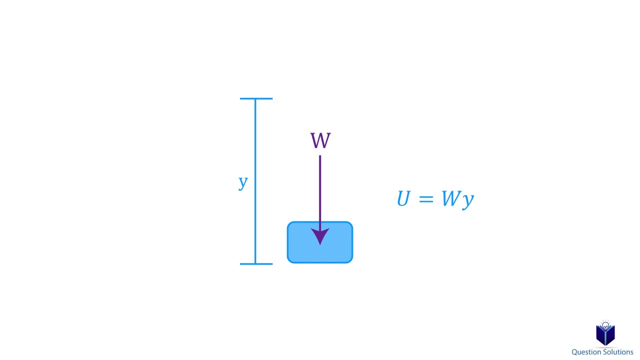 by the distance the particle traveled in the vertical direction. We say the work done by weight is positive when the particle moves downwards. Now that we got work covered, we can head into the big equation, which is this: It's t1 plus sigma u is equal to t2.. 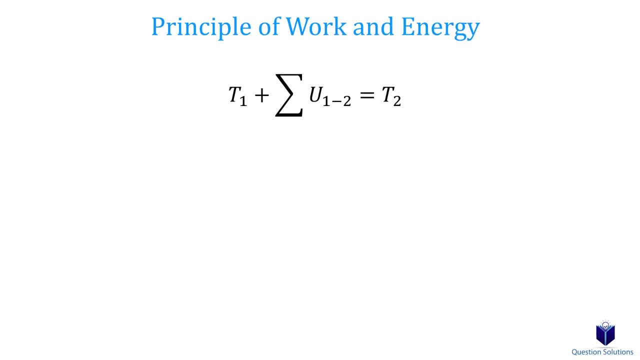 This is called the principle of work and energy. It means very little like this, So let's expand on it. The first, t1, represents the initial kinetic energy of a particle, The sigma u represents all the work added together and t2 represents the final kinetic. 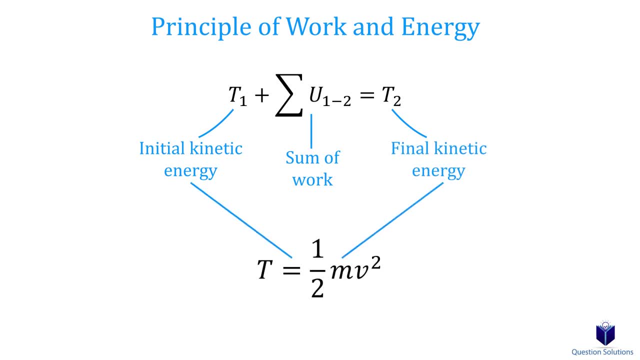 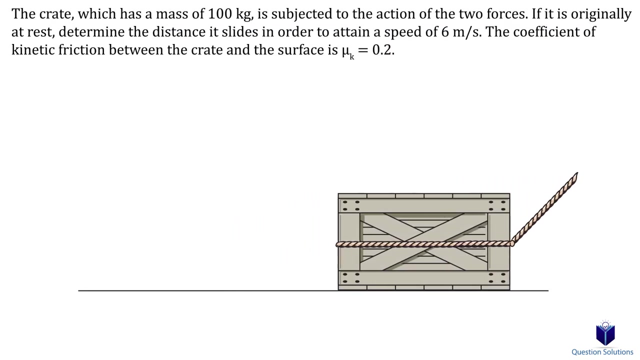 energy of a particle. Kinetic energy is half times the mass times the velocity squared. Another way of saying this is that the initial kinetic energy of a particle, plus the work done, is equal to the final kinetic energy. When we do examples, this will make more sense, so let's get to it. 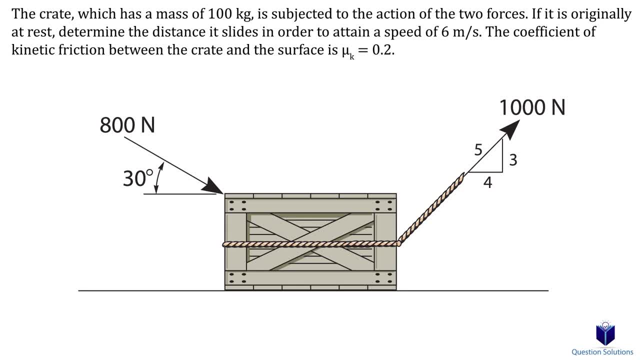 In this question. we need to find the distance. the crate slides in order to attain a speed of 6 meters per second. We're given the coefficient of kinetic friction, so we do need to consider friction in this problem. Looking at the diagram, we have two forces: one pushes and one pulls. 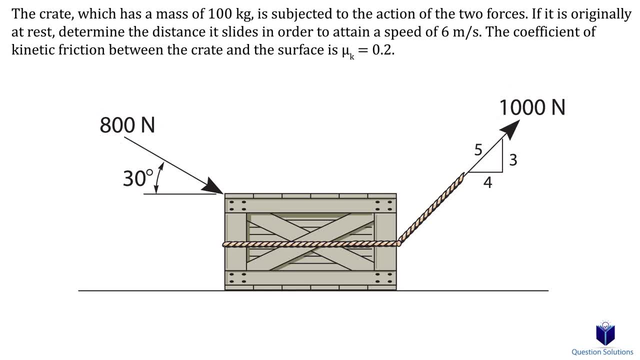 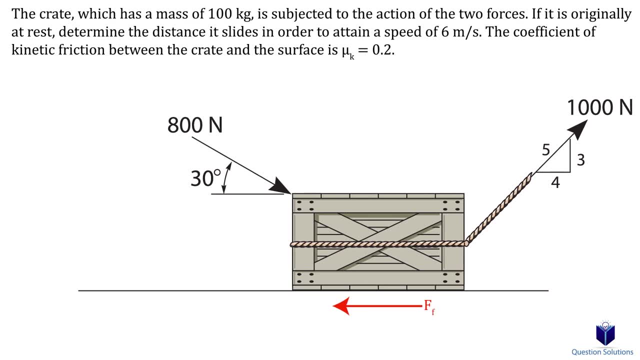 So both of those forces will do positive work, but since we're considering friction as well, the frictional force will do negative work. In simple terms, the two forces will move the box to the right, while the frictional force will try to slow it down. 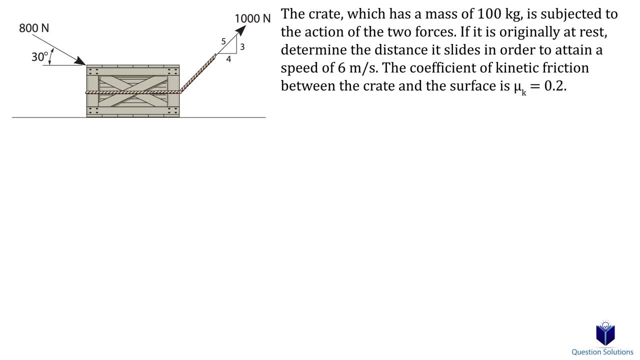 So our first step is to actually figure out what this frictional force is, And to do that, we will start off by drawing a free body diagram. So we have the two forces: the weight, the normal force and the frictional force. 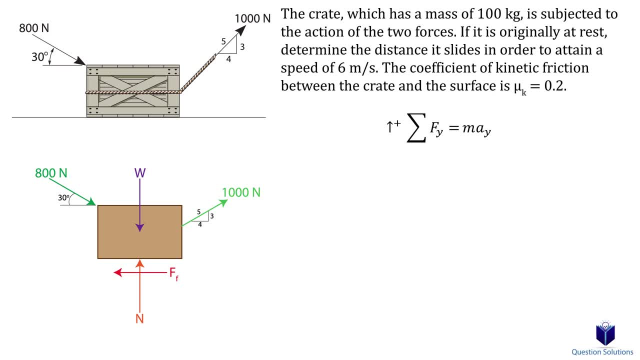 Let's write an equation of motion for the vertical direction That will allow us to find the normal force, Assuming forces upwards to be positive. we have the normal force, the weight, the y components of the two forces And that's equal to mass times acceleration. 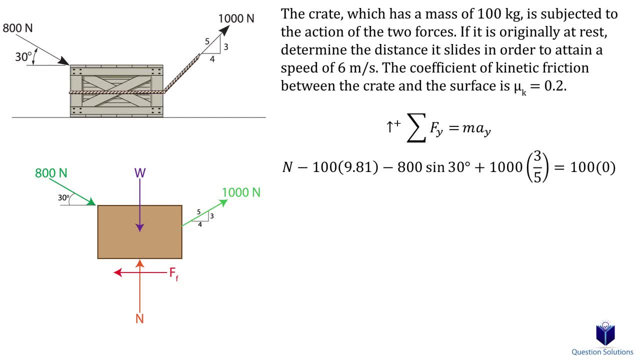 And that's equal to mass times acceleration. But remember the crate is only moving along the horizontal axis, not the vertical axis, So acceleration in the y direction is zero. Let's solve for the normal force. Now we can calculate the frictional force, which is the normal force multiplied by the 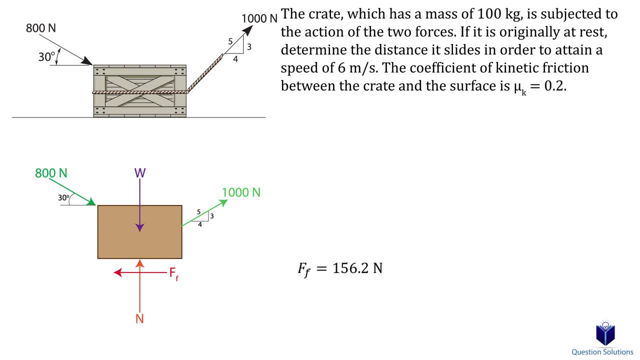 coefficient of friction. Let's think about work and energy. So the box moves in the horizontal axis, Any force that makes the box move in the horizontal axis, so the x components of the forces and frictional force will do work, Whereas forces like weight and the force will do work. 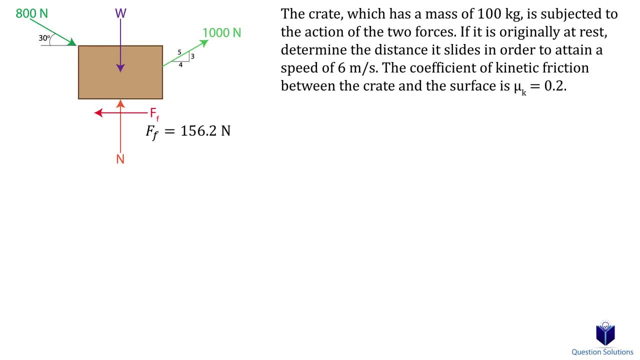 So we can write the principle of work and energy equation. So let's break down what's happening here. We got half the mass times, initial velocity, which is zero since the crate starts from rest. Then we add up all the work So we got x component forces multiplied by the distance the crate moves. 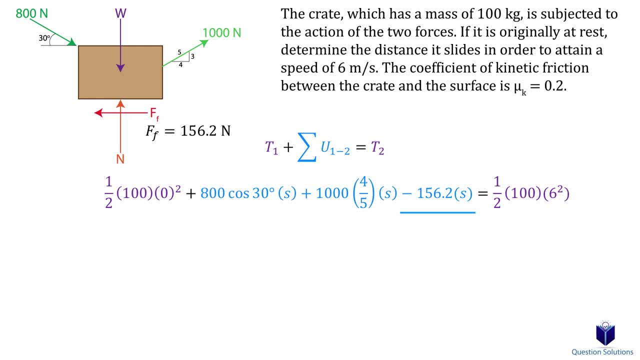 And the frictional force multiplied by the distance travelled, That's equal to half the mass times the final velocity squared, which is 6 meters squared. Now we can write the principle of work and energy equation. So let's break down what's happening here. 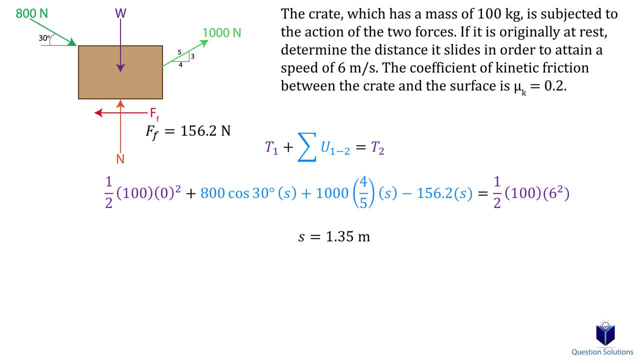 We got half the mass times initial velocity, which is zero since the crate starts from rest. Then we add up all the force multiplied by the distance travelled, So we get half the mass times initial velocity squared, which is zero since the crate starts from rest. 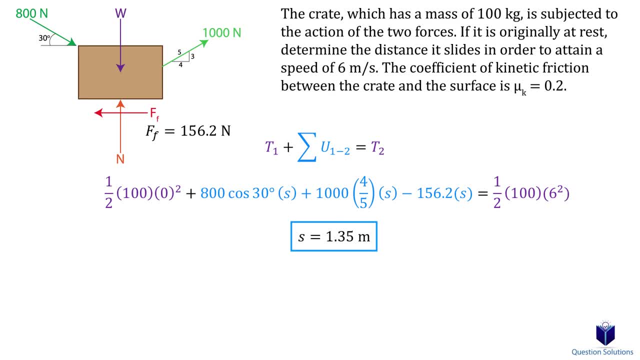 And the frictional force multiplied by the distance travelled. That's equal to half the mass times the total velocity squared. And that's equal to half the mass times the total velocity squared, We can solve for S, which is our answer. So to gain a speed of 6 meters per second, the crate slides a distance of 1.35 meters. 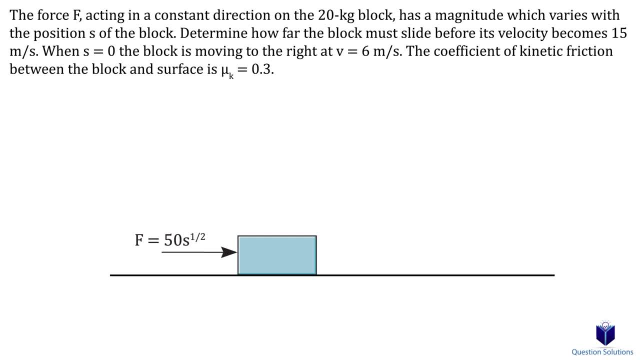 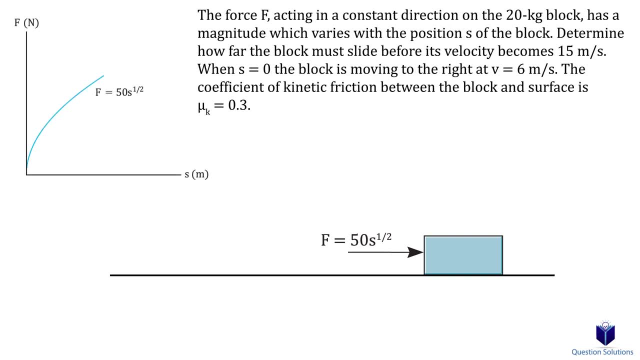 Let's take a look at this example. In this example, we need to find how far the block must slide before reaching a velocity of 15 meters per second. You should notice that, unlike the previous question, we have a variable force. The force f is dependent on the distance travelled by the block. 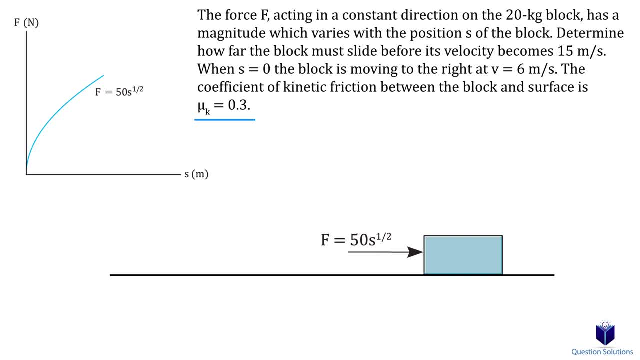 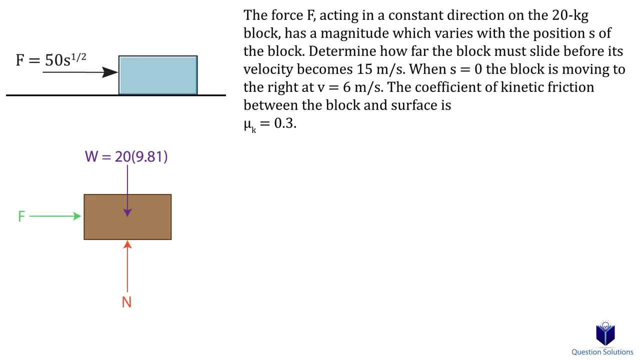 We also have friction, frictional force is. To do that we need to draw a free body diagram. So we have the weight normal force, the variable force and the frictional force. Let's write an equation of motion for the vertical forces, Since the variable force has only an x component, the only force 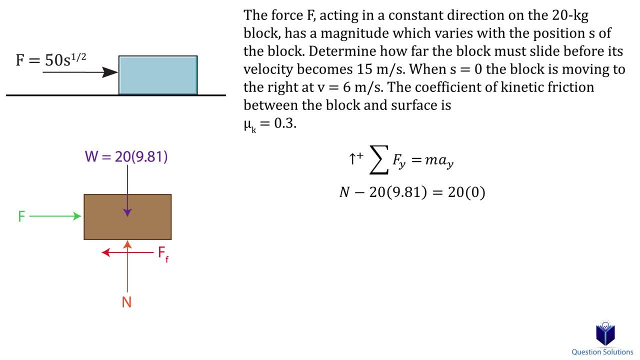 affecting the block in the vertical direction is weight and normal force. That's equal to the mass times acceleration, but the box is only moving in the horizontal direction, so there is no acceleration in the vertical direction. Let's solve for the normal force. Now we can find the. 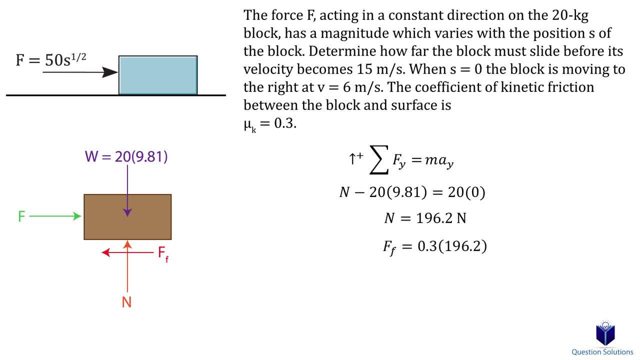 frictional force by multiplying normal force by the coefficient of kinetic friction. Let's think about work and energy. Since this involves a variable force, we will have to integrate. Keeping that in mind, let's write our equation of work and energy. So we have half the mass times, the initial. 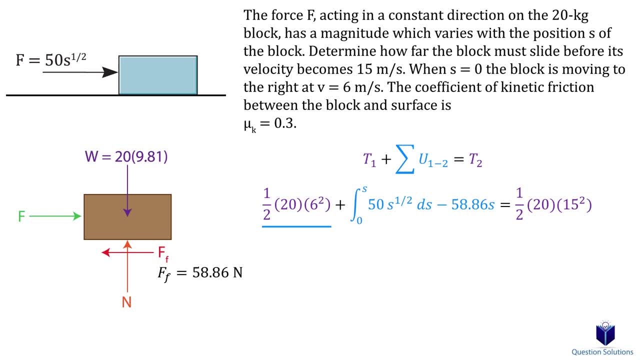 velocity. then we add all the work that's being done. together That means we have the variable force and since it's not a constant, we have the work and energy. So we have the work and energy constant. we will integrate it from a starting position of 0 meters to s. s is the total distance. 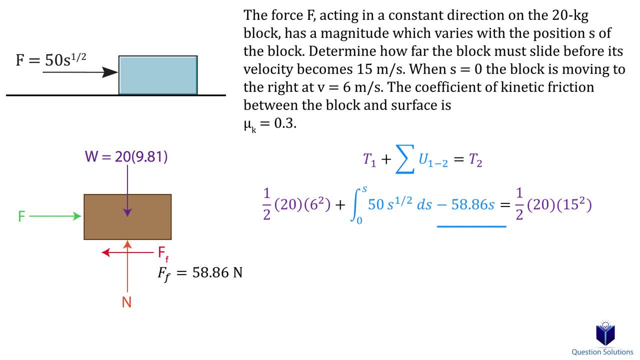 the block travels. We also have the friction, which is then multiplied by the distance traveled. All of that is equal to half the mass times, the final velocity Going back to all the work being added together. remember, only x component forces will do any work. So forces like weight and the 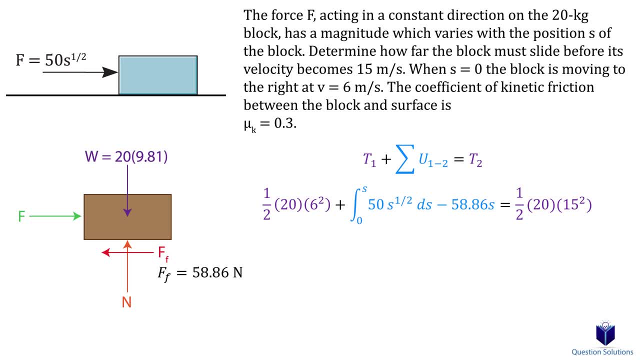 normal force will not do any work for the block because it's not moving in the vertical direction. Let's simplify and solve the integral. Now we can write the integral of x component. by the integral of x component, We can solve for s, and that's our answer. Let's take a look at this question involving pulleys. 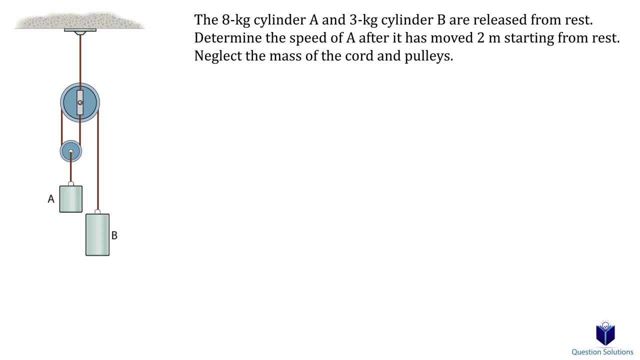 In this question we need to find the speed of cylinder A after I move 2 meters from rest. So, as with pretty much every pulley problem you face, the first step is to draw a datum. We can place it on the top pulley, Then we draw our position coordinates. We have sA and sB. 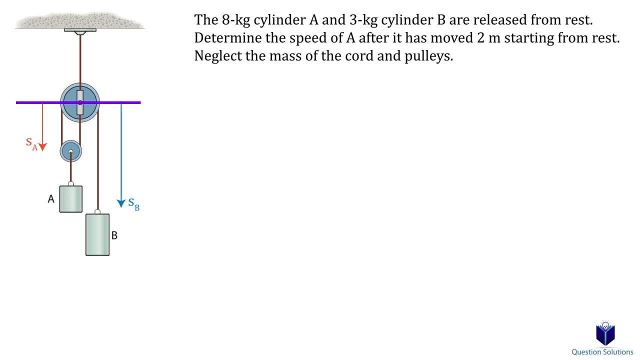 Looking at the diagram, it's one single cable, so we only need one equation. So we have 2sA plus sB is equal to the total length. If we consider a change in displacement, we can write that displacement using delta. The reason why we do this is because we want to figure out how much. 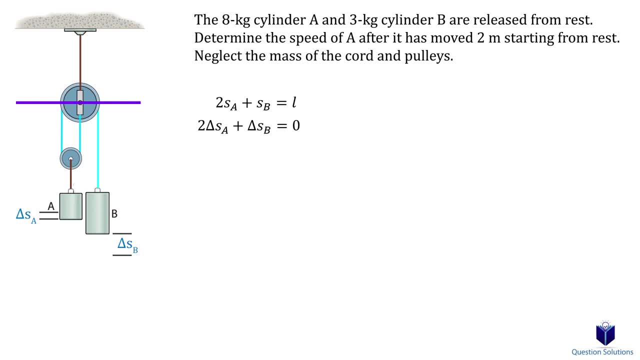 cylinder B moves when cylinder A moves 2 meters. So let's plug in 2 meters for the change in displacement for cylinder A, and then we can figure out how much cylinder B moved. We find that cylinder B moved negative 4 meters, but that just means it moved up 4 meters. We drew our position coordinates downward, and then we can write the displacement using delta. 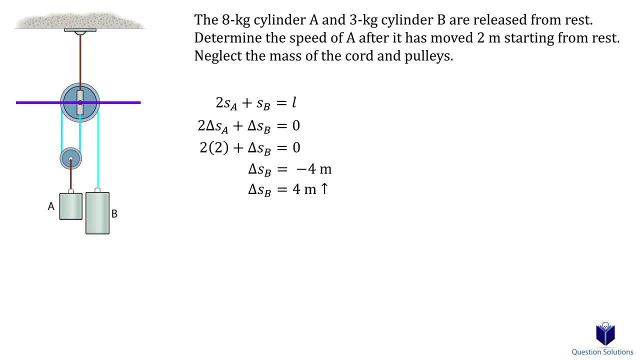 downwards, meaning any movement down was positive. Now the end result we want is to figure out the speed of cylinder A, which means we definitely need a velocity equation. So let's take the derivative of our initial equation. This equation represents the speeds of cylinders A and B. 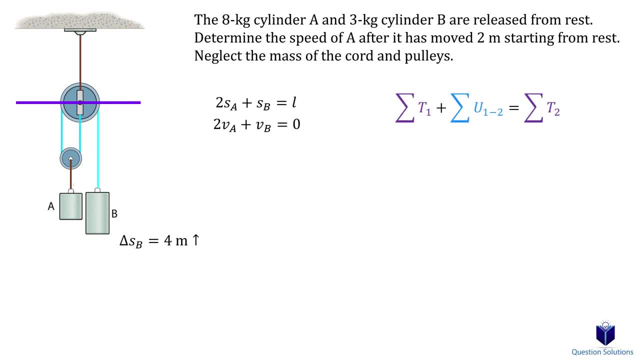 The next step is to consider work and energy. Here we think of the movements of cylinder A and B together, because their movements are tied to each other. Keeping that in mind, let's write our equation, Since it's the addition of both kinetic energies, of both. 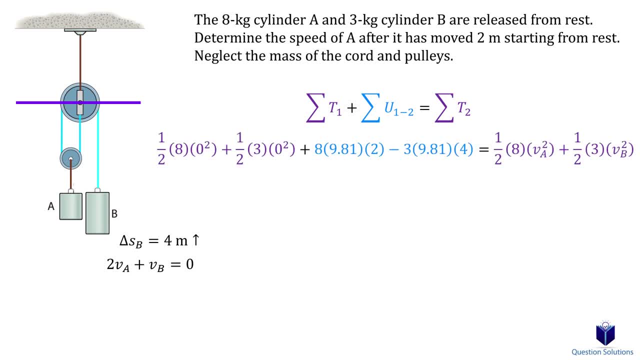 cylinders, we will add the big sigma sign in front of the t's. Let's go through this equation. For the initial kinetic energy, the system starts from rest, so all the velocities are zero. Then we have the forces that do work. 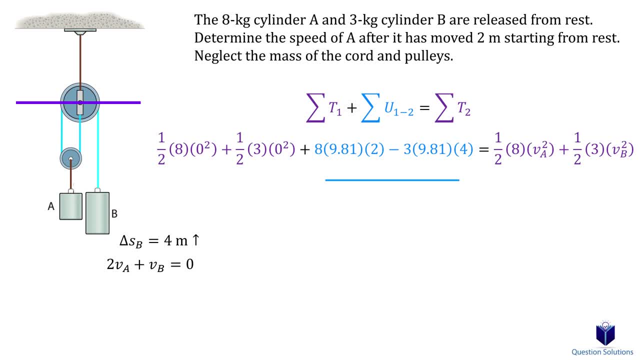 In this case that's only weight. No other force affects the system. So when we did the displacement equation we found that when cylinder A moves 2 meters down, cylinder B goes up 4 meters. It's important to note that when cylinder A moves 2 meters down, cylinder B goes up. 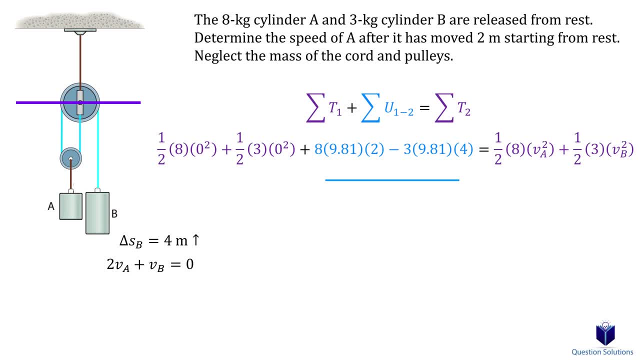 four meters to keep this in mind, because while one cylinder does positive work, the other does negative work. Again, we assume down to be positive because that's how we drew our position coordinates And since cylinder B is going up, it's going the opposite way, meaning the work that's done. 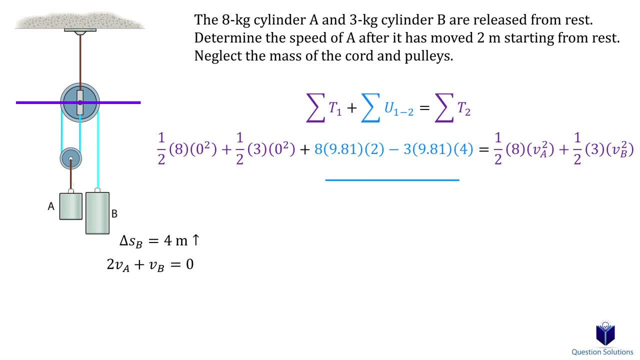 is negative. So we have the mass times, the acceleration due to gravity, multiplied by the distance traveled. On the right side of the equation we have half the mass times, the velocity of A squared, plus half the mass times, the velocity of B squared. Now we have two equations with two. 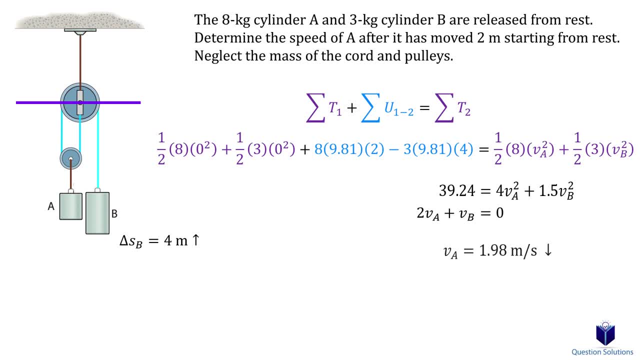 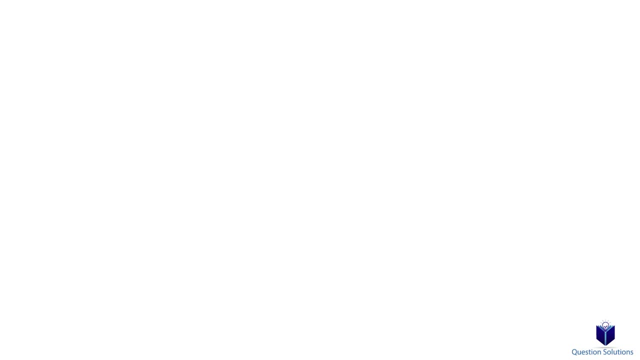 unknowns. We can solve them to figure out the velocity of cylinder A and B. So we get a negative value for B, which again simply means that it's going opposite to the way we chose it to be positive. So it's going up at a velocity of 3.96 meters per second. Let's take a look at one last. 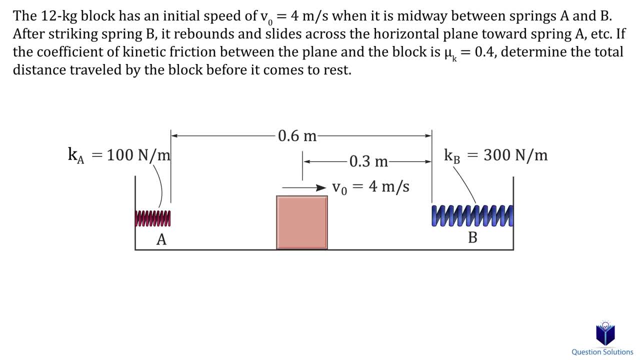 example involving springs. In this question we need to find the total distance traveled by the block. So there are two ways to approach this problem. First, we can assume that the block hits spring B, bounces back but stops before reaching spring A. OR we can assume the block hits spring b and 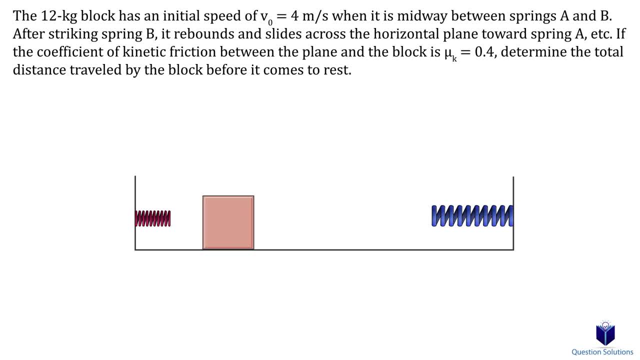 slides all the way to spring A and then comes back and stops. We will assume the first condition and see if it's true. If it is, that's less work for us. otherwise we need to recalculate the distance traveled when it reaches spring A and do another equation to see where it stops. So let's start off. 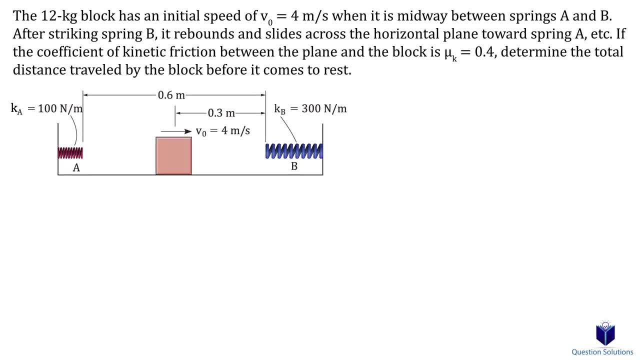 by first figuring out the frictionaling equation for the block force. For that we can draw a free body diagram of the block. So we have the normal force, the weight and the frictional force. Let's write an equation of motion for the vertical motion. 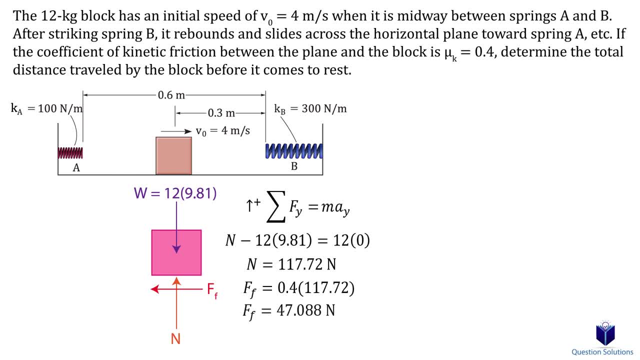 Let's solve for the normal force, and now we can figure out the frictional force. Let's get started with our equation of work and energy. The block will slide towards spring B, compress it and stop. Our first goal is to figure out how much distance the block travels. 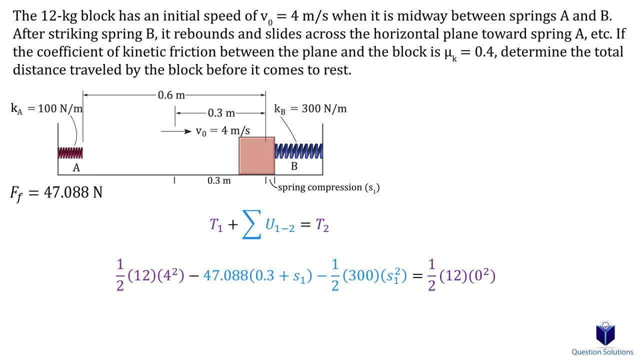 In other words, how much does the spring compress? because the total distance that the block travels is 0.3 meters plus the distance the spring compresses. So first we have half the mass multiplied by the initial velocity, then we have the work that's being done. 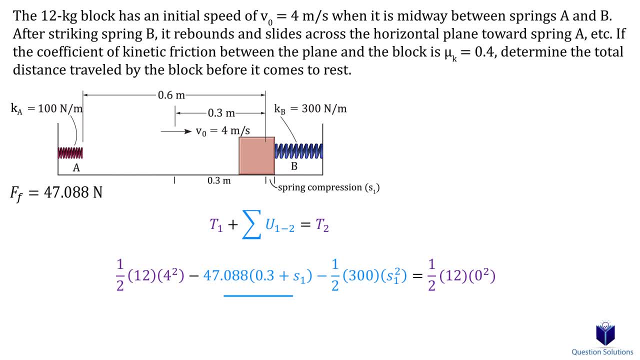 We have the frictional force which is doing negative work. So the block travels a total of 0.3 meters, plus the distance it compresses the spring, Remember, even while the spring is being compressed the block experiences friction. So the total distance that the block travels, 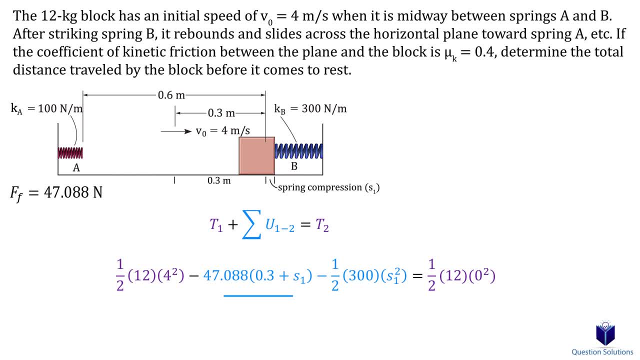 before it stops is 0.3 plus S. S is the distance the spring compresses. Then we have the spring, which also slows the block down until it stops. so it does negative work. So that's half times the stiffness of the spring multiplied by the displacement. squared, All of that is equal to: 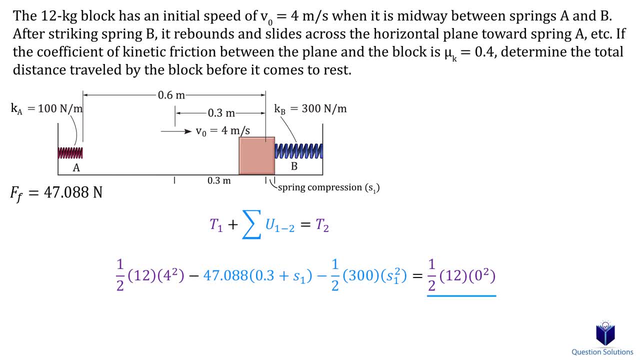 the final kinetic energy, which is zero because the block is no longer moving Again. S represents the distance the spring compresses before stopping the block. Now the spring is being compressed so it's doing negative work. So the block is moving, but the spring is pushing back the block. 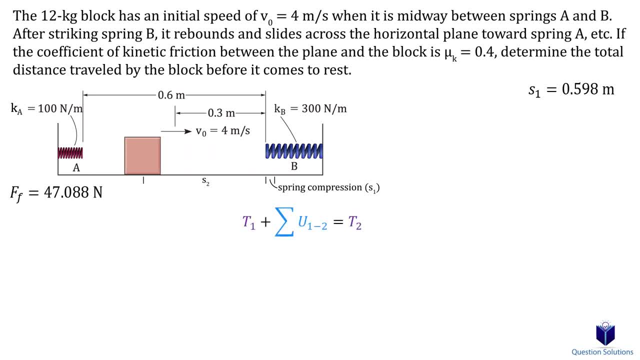 in the opposite direction. So we write another equation for work and energy. This time the spring is actually doing positive work, while the friction is still doing negative work. Remember, we're trying to figure out where the block will stop now. So the initial and final velocities. 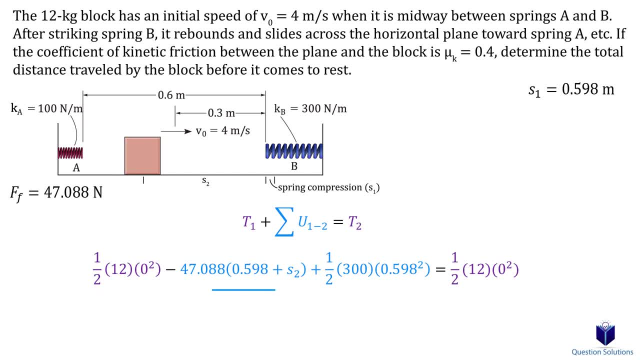 are both zero. So our initial kinetic energy is zero because the block starts from rest. Then we have the frictional force doing negative work while the spring is doing positive work. So we have the frictional force doing negative work while the spring is doing positive work. 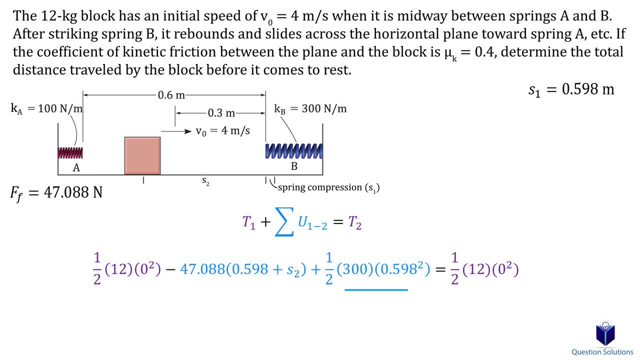 So we have 0.598 meters. and for the frictional force, remember that in addition to the compressed distance the block travels, it will go S meters until it stops. So S in this equation is the distance the block travels before stopping. Then, on the other side, we have the final kinetic. 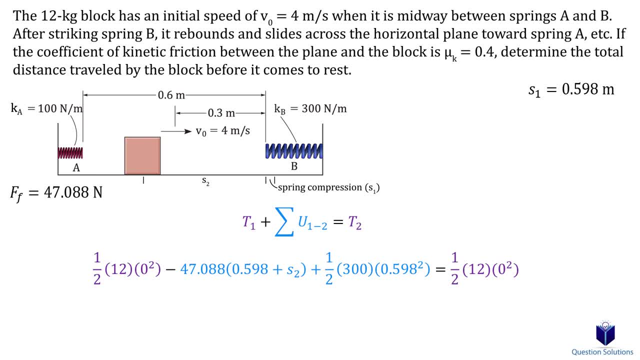 energy, which is zero, since the block comes to a rest. Let's solve for S, So that's the distance the block travels before stopping, since that's less than 0.680 meters, So we have 0.598 meters. the block doesn't hit spring A, So we don't need to do any more calculations.